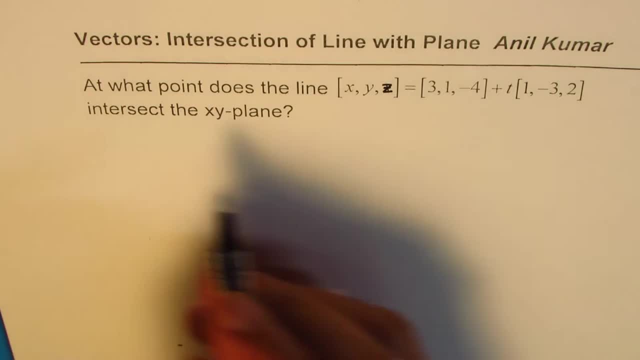 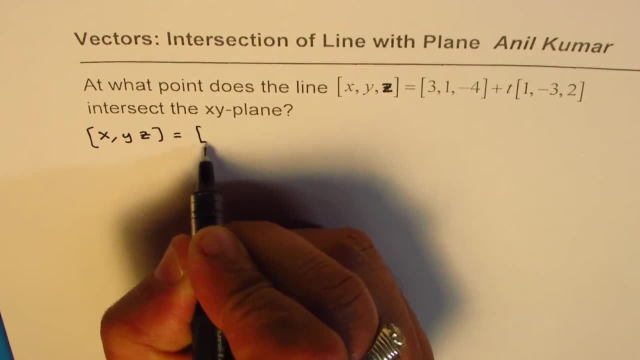 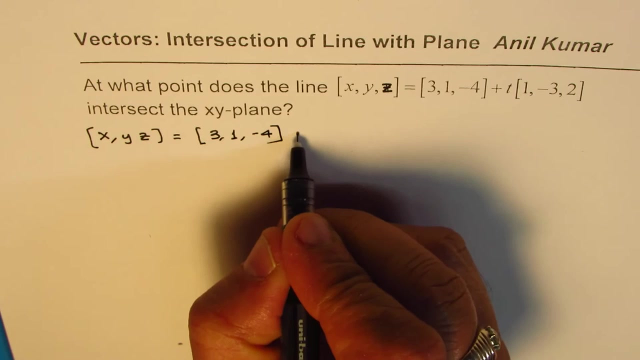 question and then look into my suggestions. Well, the vector equation is given to us. It is x, y, z equals to 0.3, 1, minus 4.. That's the position vector t times 1, minus 3, 2.. 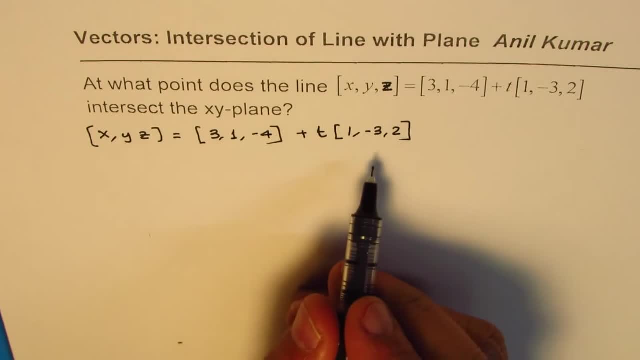 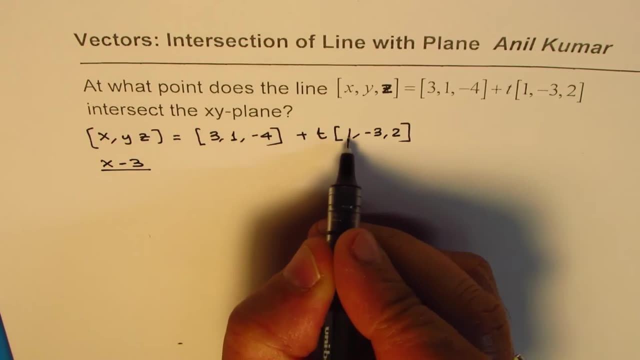 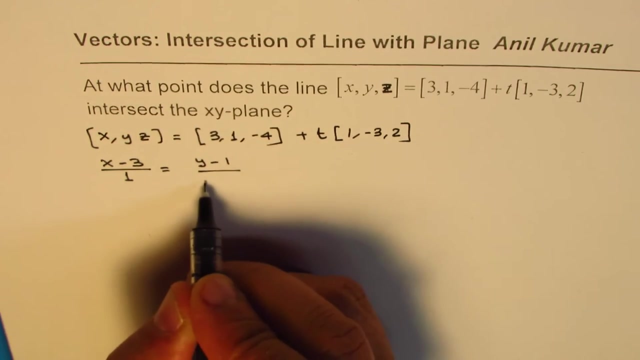 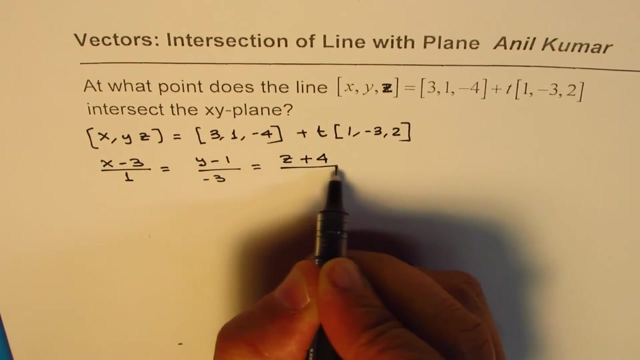 And that is the direction vector. Now, from this equation we can always write the symmetric equation, Which will be x minus 3, divided by 1.. So I'm just writing 1.. It is not required. y minus 1, divided by minus 3, equals to z minus Minus 4, makes it plus Plus 4, divided. 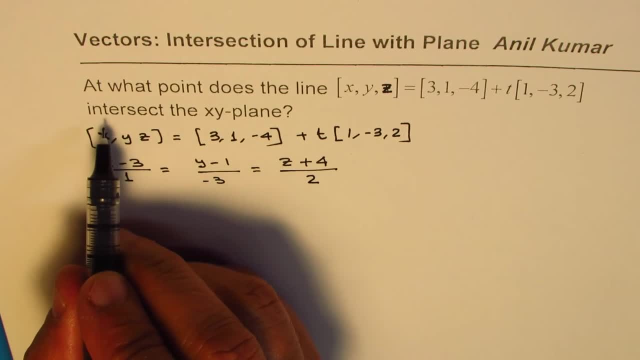 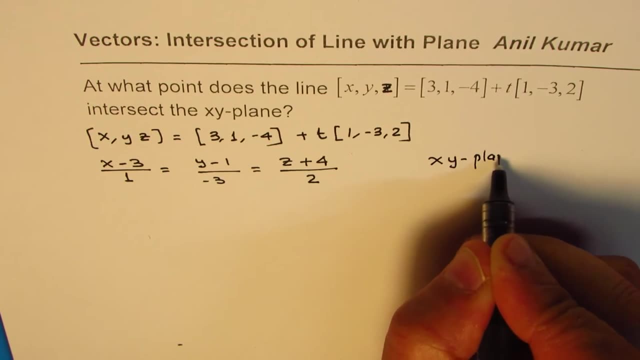 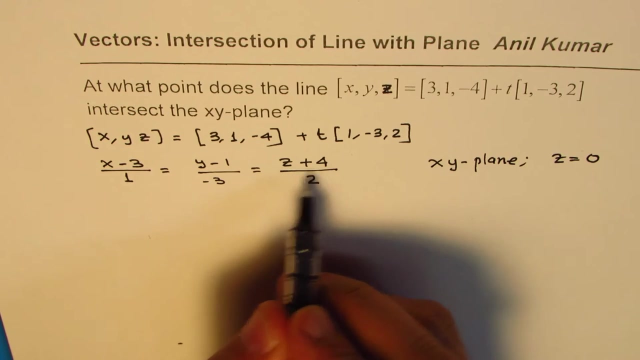 by 2.. Now if you want to find intersection with x y plane, right. So x y plane means what? It means that z should be equal to 0, right? So if I substitute z equals to 0 in this. 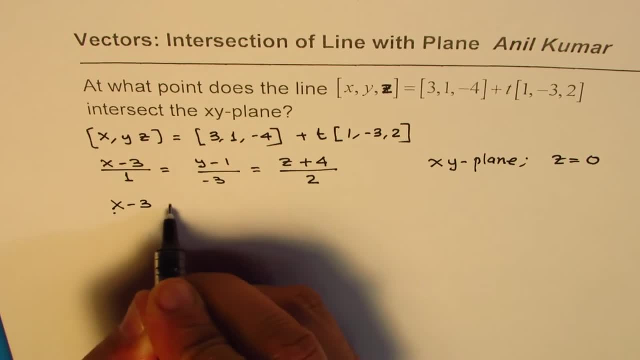 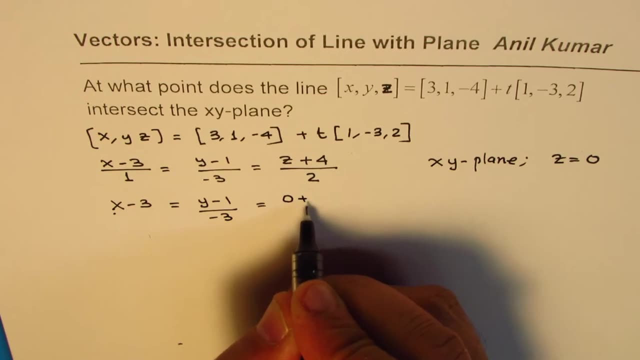 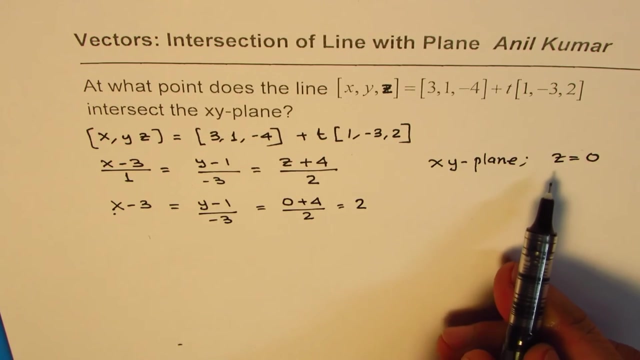 equation. what do I get? I get x minus 3, equals to y minus 1, over minus 1, equals to 0, plus 4, over 2, which is actually 2.. So we know that z is 0.. We can find x and. 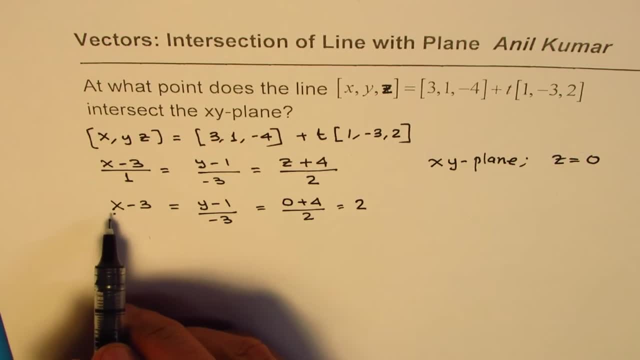 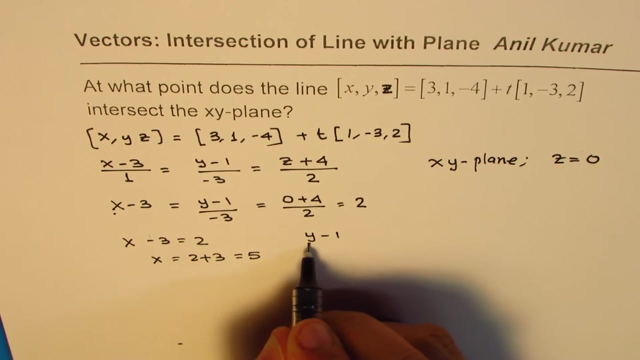 y points right. So values. So x is equals to. so we have x minus 3 equals to 2.. That means x is equals to 2 plus 3, which is 5.. As far as y is concerned, y minus 1, over minus 3, equals to 2.. Y minus. 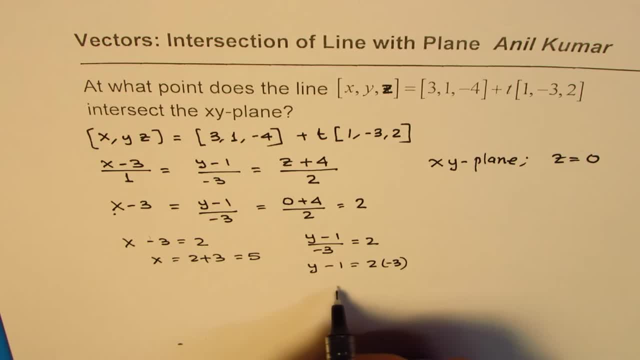 1 is equals to 2 times minus 3.. And y is equals to 2 times minus 3, plus 1,, which is 2.. So there is a point here. So y is equal to both of those points and z is equal to 3.. 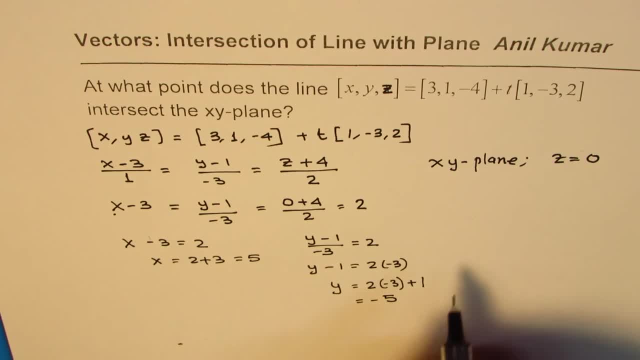 We have that point: x minus 1 over 2, that is the intersection. So 2 times minus 3 is equal to minus 6, which is minus 6, which is minus 5.. So what is the point of intersection? Well, the point of intersection.